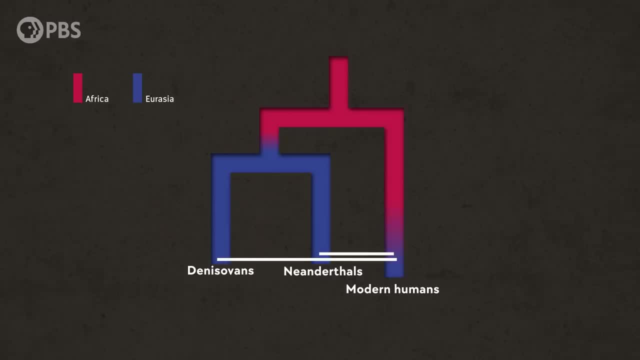 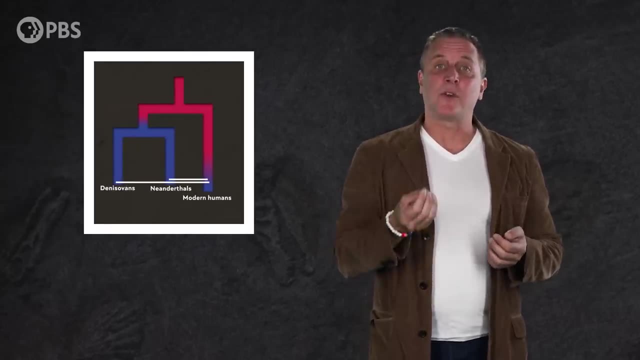 There they met and interbred with other hominins that already lived there. our ancient cousins, the Neanderthals and Denisovans, And all living people of non-African descent come from those migrants. so bits of Neanderthal and Denisovan DNA can still be found in our gene pool today. 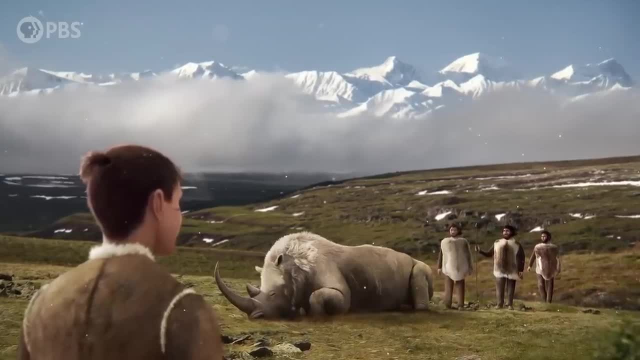 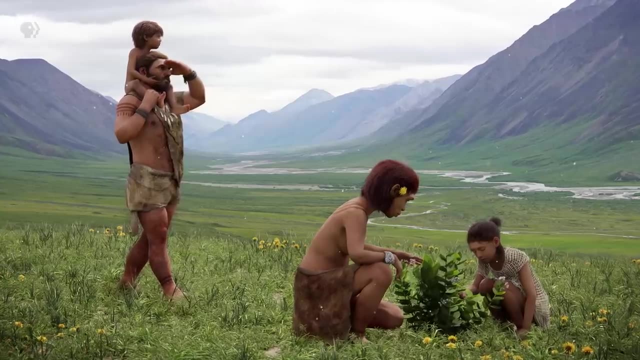 We talked about this in our episode called When We Met Other Human Species, But now we want to flip the script. What happened when these ancient cousins met us From the Neanderthal side? only a small percentage of their total DNA can be traced back to interbreeding with us. Overall, they were much more similar to Denisovans. 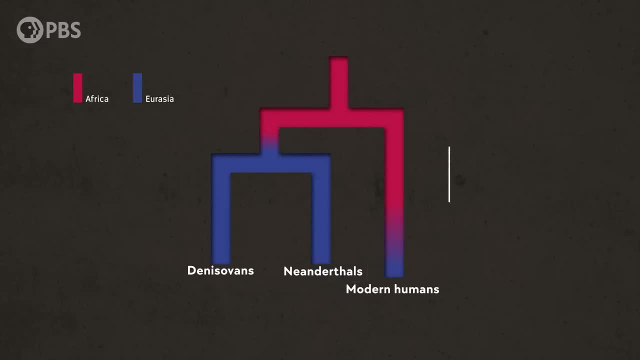 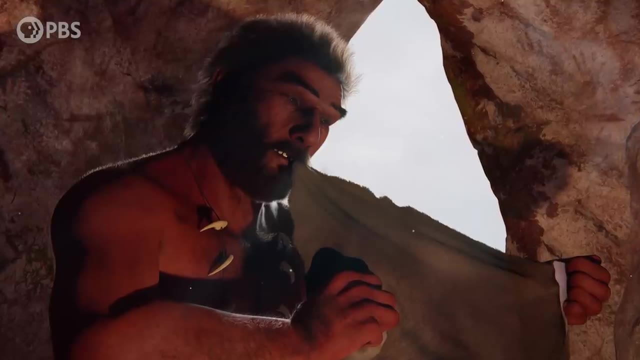 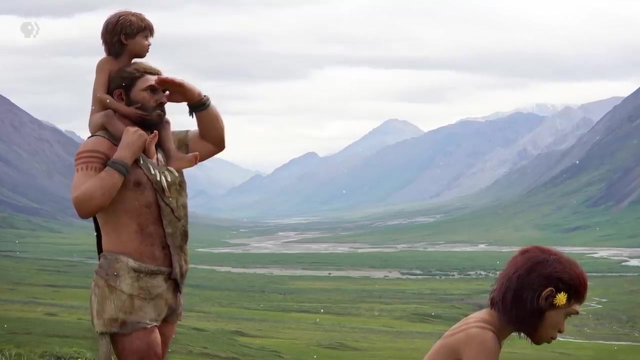 because they were each other's closest evolutionary relatives. So the fact that the Neanderthal Y chromosome was more like ours than the Denisovans was a surprise One that suggests that the whole thing was completely replaced in what seems to be all-male Neanderthals. But when did this Y chromosome replacement happen, and why? 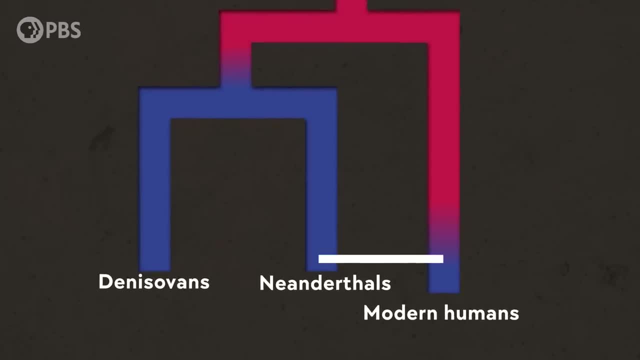 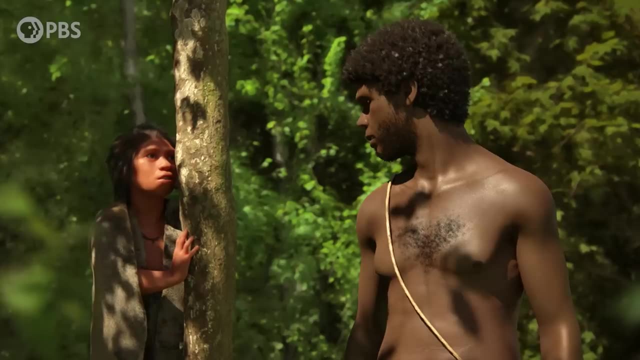 The interbreeding events that took place around 80,000 years ago and after can't explain where Neanderthals got a human-like Y chromosome. We'd have to look much further back in time. Scientists have known that there were multiple human dispersals out of Africa. 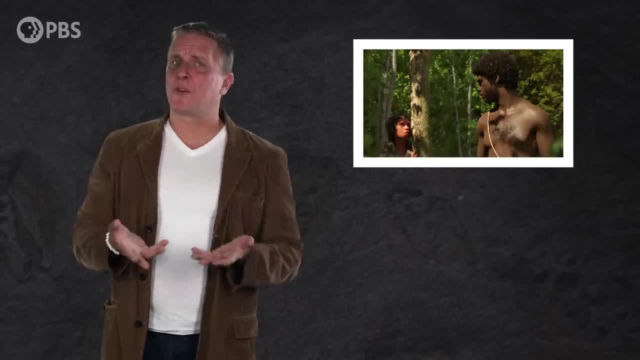 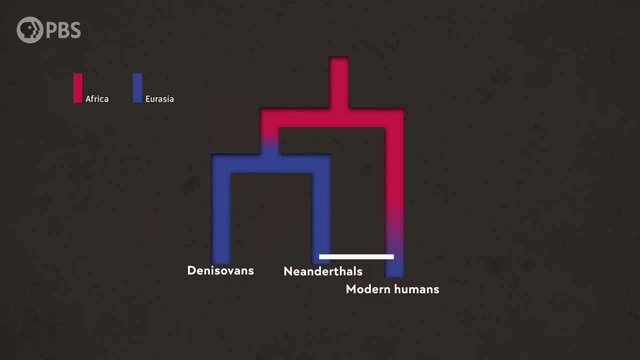 some of which didn't leave modern descendants. And we still don't fully understand these ancient interactions between different hominins and the implications of those meetings, But the Y chromosome replacement points to one of them. The researchers calculated that the human-like Y chromosome entered the Neanderthal gene pool well before the migration out of Africa. 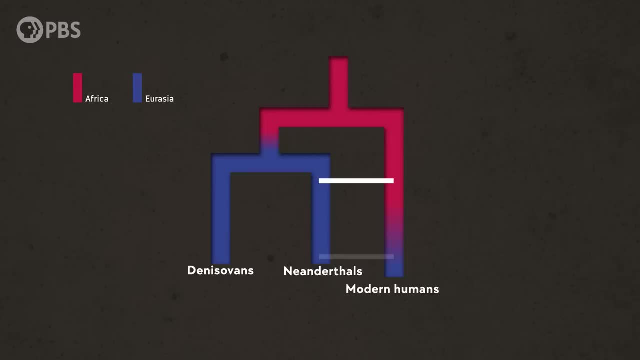 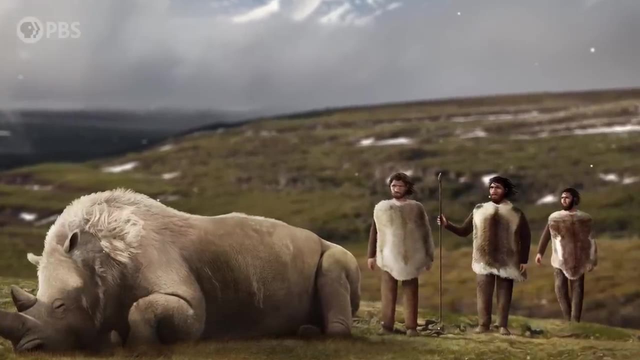 around 80,000 years ago, probably as much as tens or hundreds of thousands of years before it, Which means that many of the Neanderthals that those migrants encountered already had human-like Y chromosomes. Now, this was a really strange pattern. 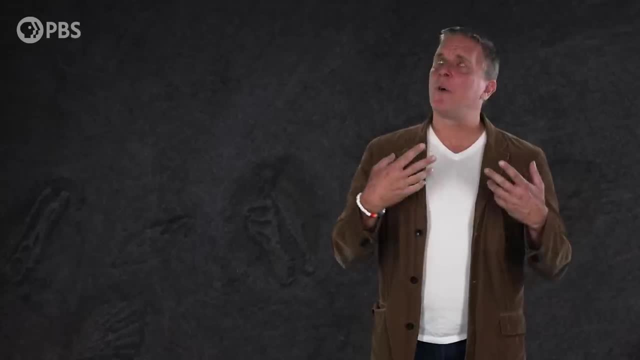 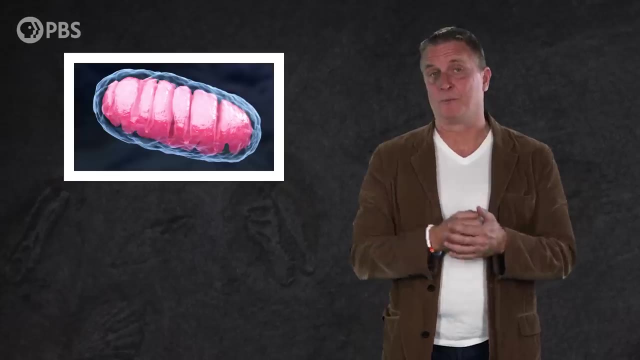 unlike what we see in any of the other Neanderthal chromosomes, But it wasn't entirely unique, See, the researchers realized that a weird pattern had recently been found in their mitochondrial DNA too. Mitochondrial DNA is a small, separate second genome that is passed down only from the mother. 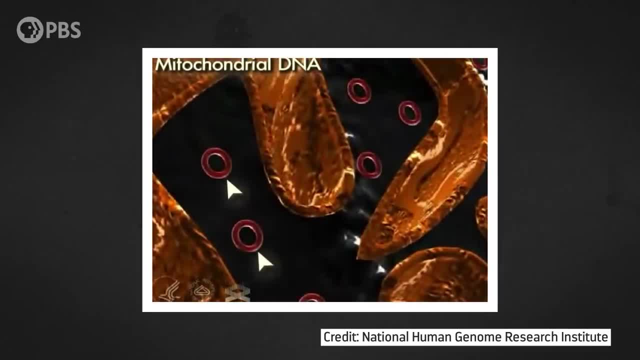 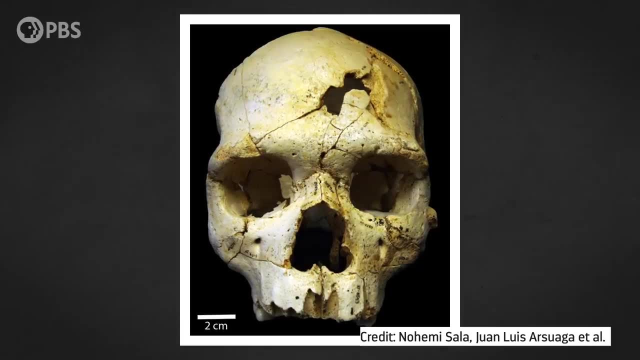 And in Neanderthals it also shows a puzzling link with ancient Homo sapiens. The oldest Neanderthal mitochondrial genomes we have come from fossils found in Spain dating to around 430,000 years ago, And their mitochondrial DNA looks very Denisovan-like. 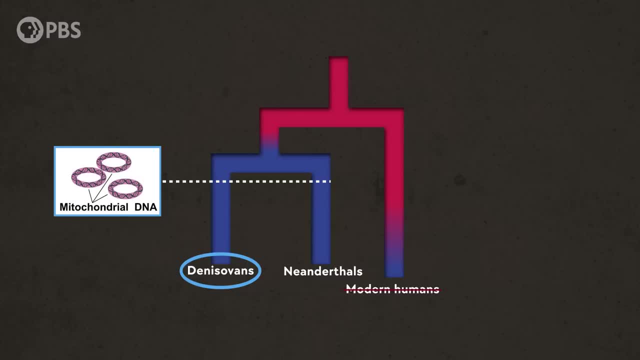 rather than human-like. This is what we'd expect based on their evolutionary relationship, But in later Neanderthals this all changes. The original Denisovan-like mitochondrial DNA is missing from all the younger Neanderthals that we've sequenced. 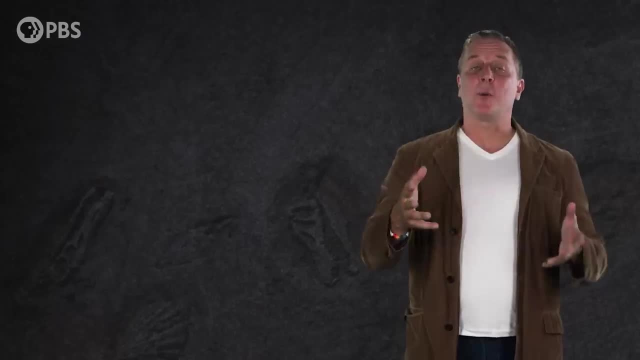 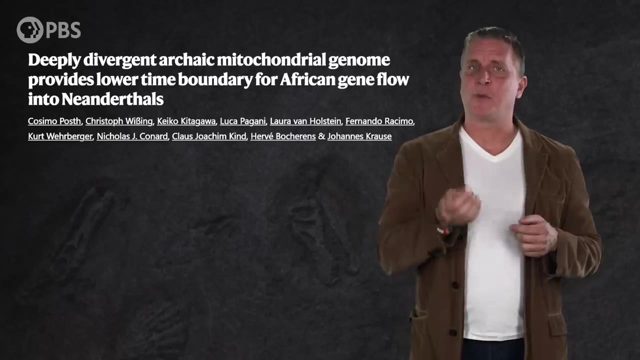 It's been replaced with DNA that's much more human-like And in 2017, it was proposed that the best way to explain this change is a previously unknown period of very early gene flow: Neanderthals and ancient Homo sapiens. Neanderthals and ancient Homo sapiens. 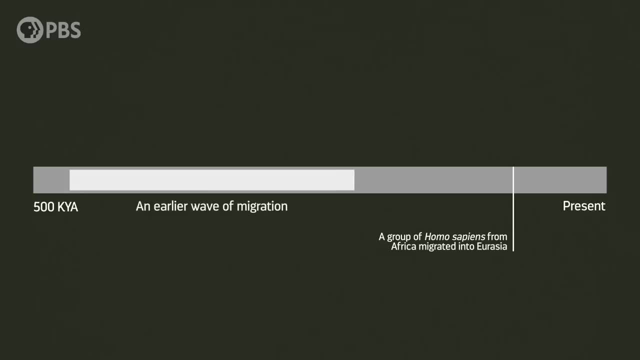 Specifically, sometime between 470,000 years ago and 220,000 years ago, a wave of ancient Homo sapiens from Africa, or a group closely related to them, migrated into Eurasia, While this wave eventually died out without leaving any direct descendants in modern-day. 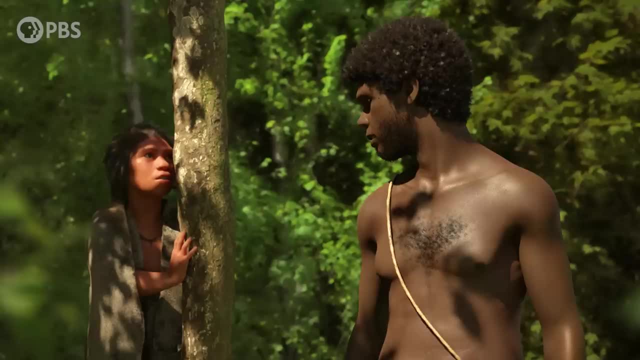 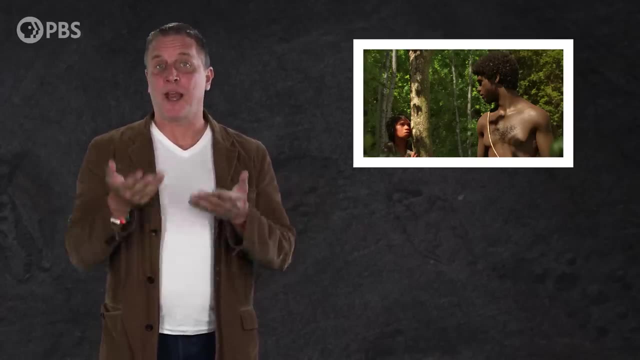 populations, they did leave a genetic legacy behind. in Neanderthals, At least one female individual from that group reproduced with a male Neanderthal, and their hybrid offspring inherited her mitochondrial DNA. Neanderthals and ancient Homo sapiens. Neanderthals and ancient Homo sapiens. 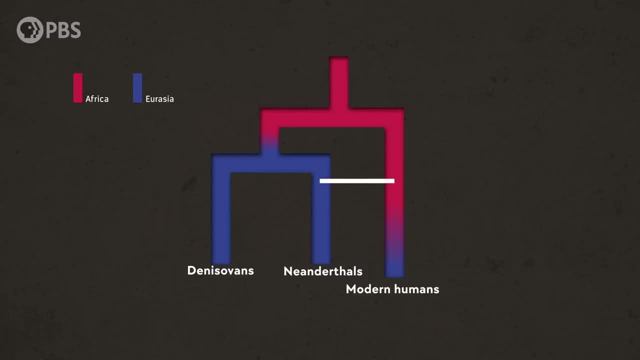 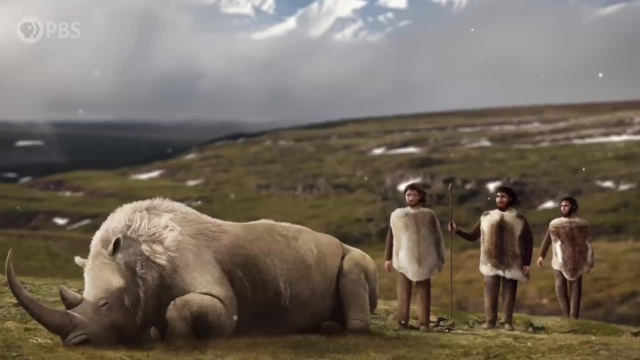 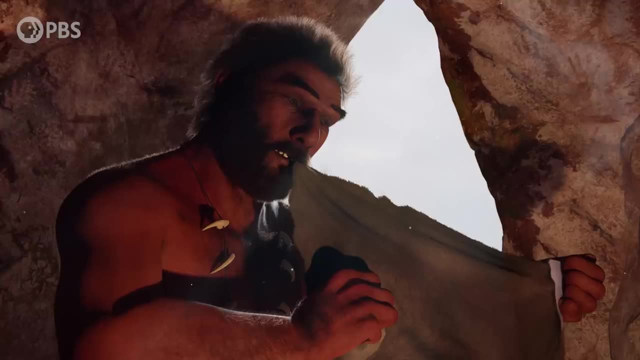 mitochondrial DNA through the Neanderthal gene pool, Eventually over tens to hundreds of thousands of years. this mitochondrial DNA seems to have completely replaced the original delisivin-like mitochondrial DNA in Neanderthals. So when the researchers later found human-like 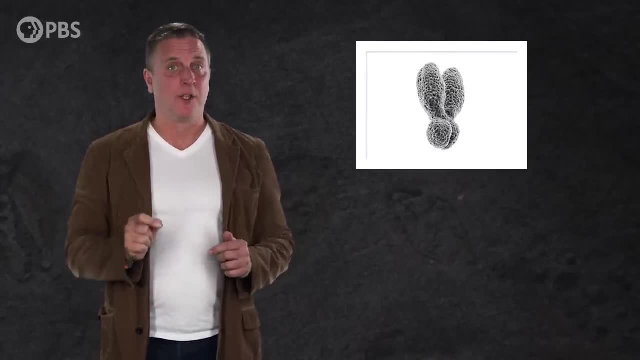 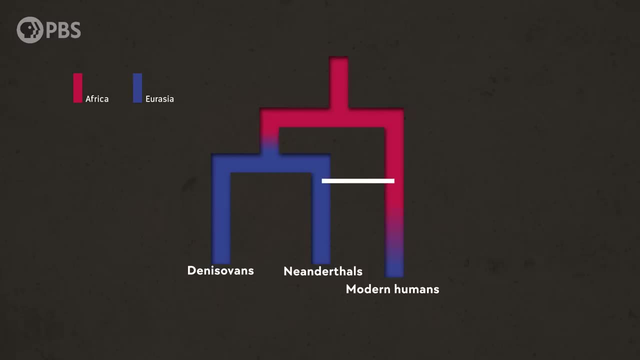 Y-chromosomes had also taken over the Neanderthal gene pool, they realized it must be a piece of evidence for very early periods of interbreeding. The only real difference is that in this case at least one human male had sons with a female Neanderthal. 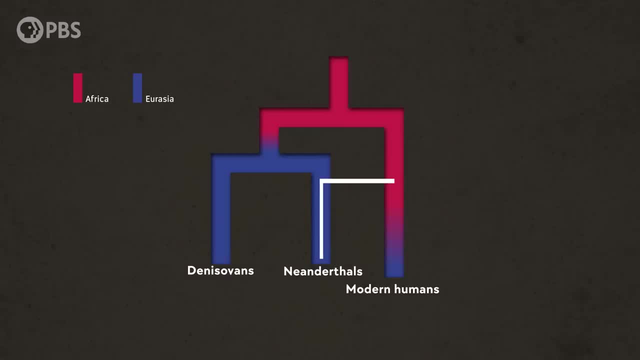 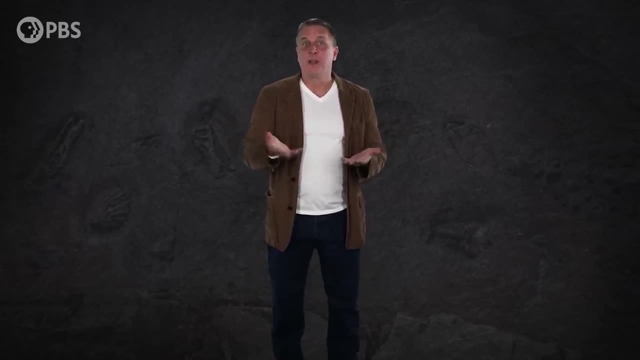 introducing his Y-chromosome into the Neanderthal gene pool via those male hybrid offspring. Now for us to actually confirm that the early gene flow is behind the Y-chromosome situation, we'd need to find the same evidence that we have for the mitochondrial DNA, Namely 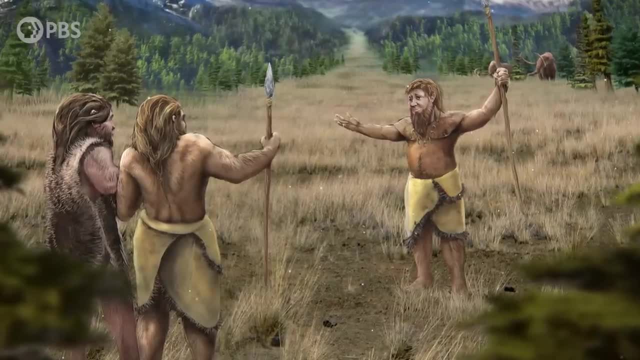 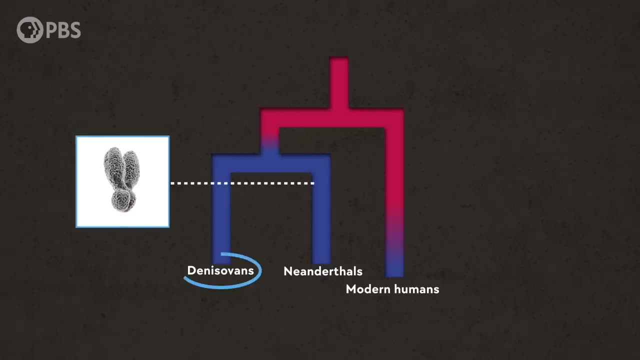 we'd need to sequence some really old male Neanderthals that predate any gene flow with ancient Homo sapiens. If and when we manage that, we'd expect that their Y-chromosomes would be like the original version, the one that looks more like the delisivin version than ours. 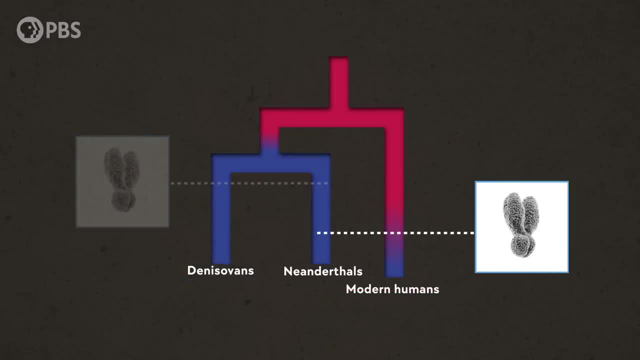 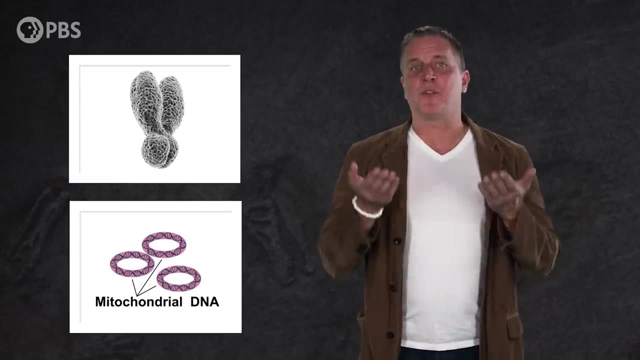 So right now we only have the replacement Y-chromosome, not the one that was replaced. Okay, but why did the human mitochondrial DNA and Y-chromosome end up totally pushing out the ancestral Neanderthal versions? After all, it's not like we see this happen in just a few Neanderthal. 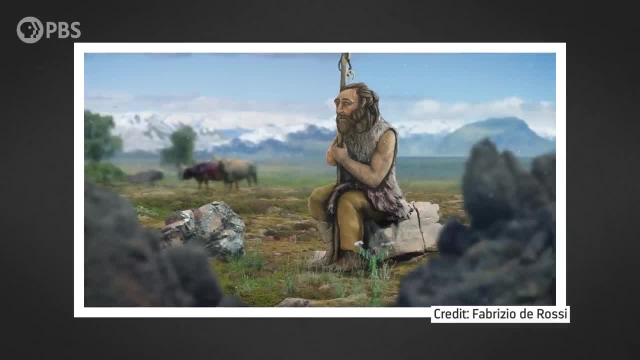 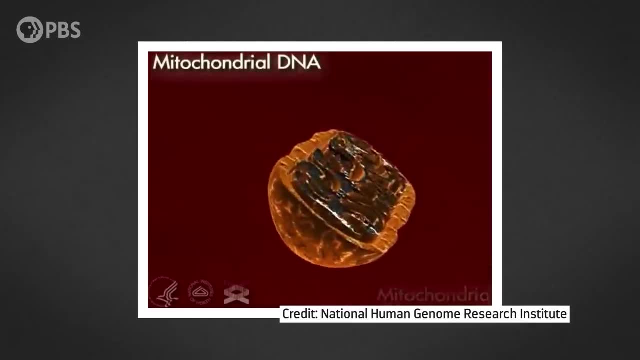 lineages in a couple of locations. As far as we can tell, all Neanderthals eventually ended up with them. If there were parallel replacements to have occurred, they must have provided some kind of fitness advantages over the Neanderthal versions. Now we don't know exactly what those advantages were, but we do have a good idea about why ancient Homo sapiens DNA might have had an edge, and it all comes down to population size. See, in small populations, natural selection is way worse at weeding out harmful mutations. 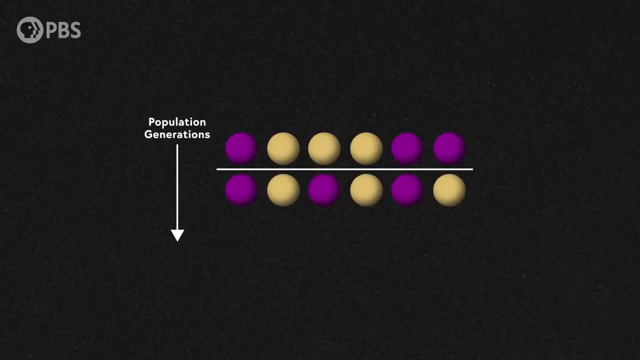 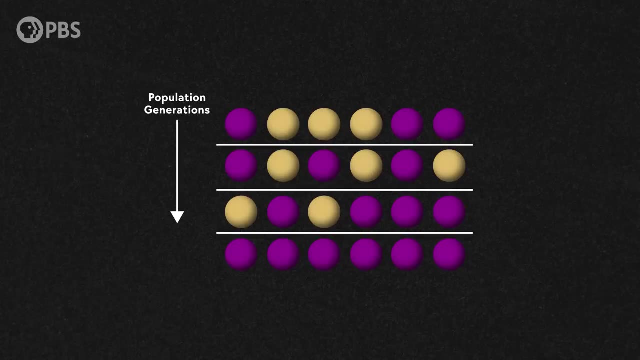 so they build up at a faster rate than in bigger populations. all else being equal, And it's been argued for a while, based on both fossil and genetic evidence, that Neanderthal population sizes were pretty small, probably for a long time, Which means that their Y-chromosomes and 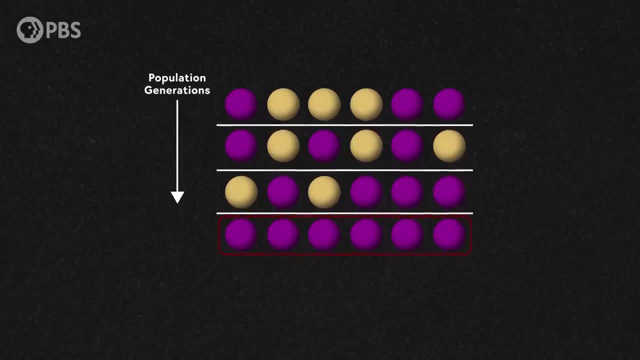 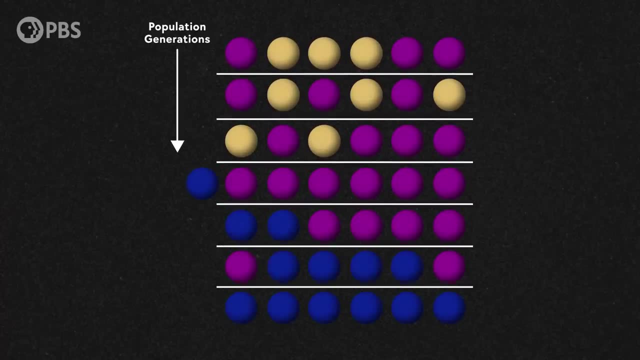 mitochondrial genomes probably had a higher buildup of harmful mutations. So as soon as ancient human versions were introduced, they were immediately favored by natural selection and rapidly spread through the Neanderthal gene pool. As for why we don't see similar replacements in the Denisovan gene pool, well, it probably. 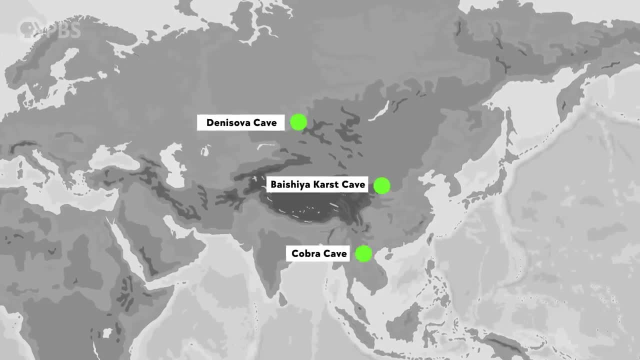 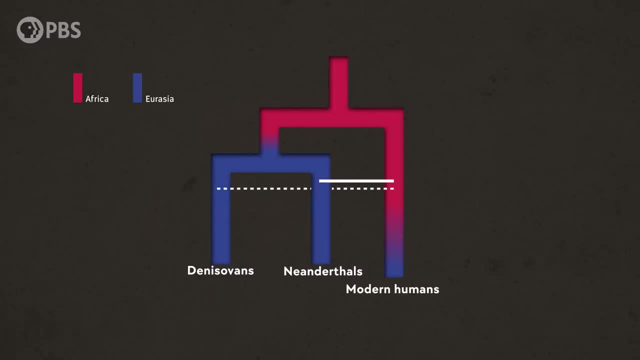 just came down to distance. They lived much further away than the Neanderthals and were concentrated in Asia and Oceania as far as we could tell. So there would have been less gene flow between ancient Homo sapiens and Denisovans during those. 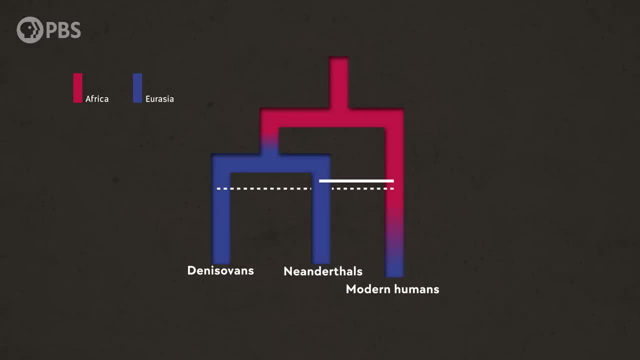 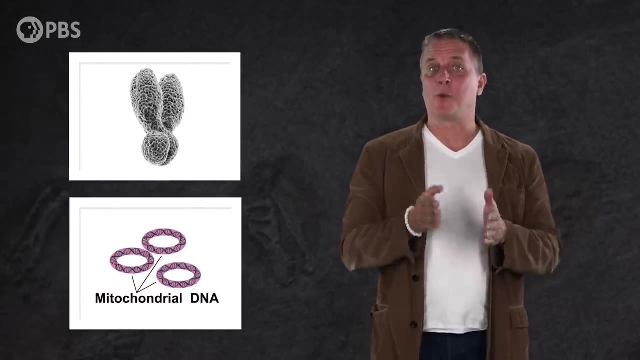 early waves of migration, certainly much less than with Neanderthals who lived in the Middle East and Europe Together. the Neanderthal Y-chromosome and mitochondrial DNA are two new lines of evidence that point to a much more complex and ancient relationship between us and our 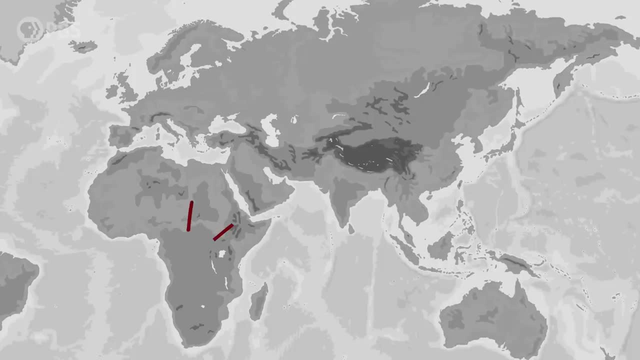 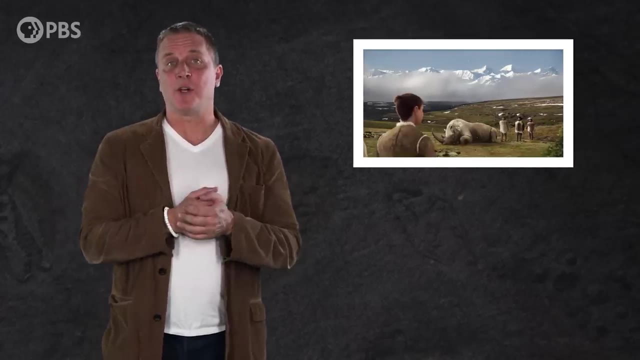 closest cousins than we otherwise would have known. They hint that the out-of-Africa migration was only one of several waves of ancient human dispersals into Eurasia, And when that successful migration happened around 80,000 years ago, it was only the latest in a series of encounters. 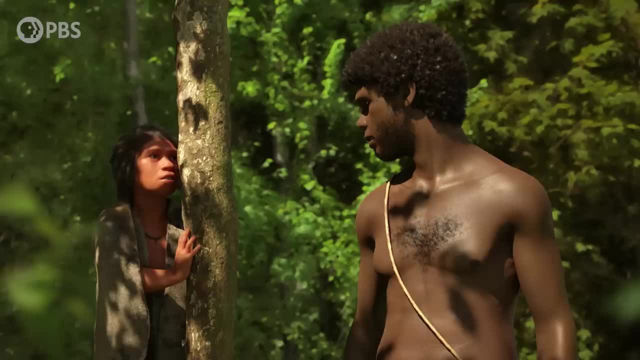 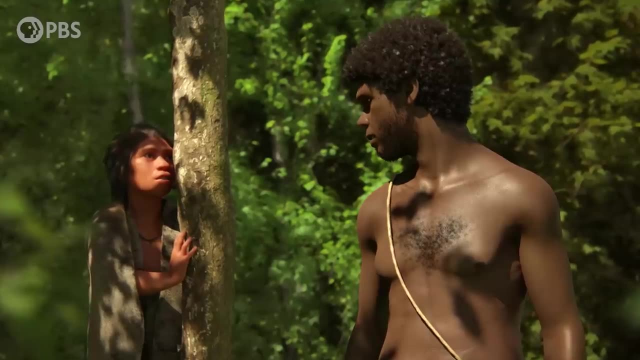 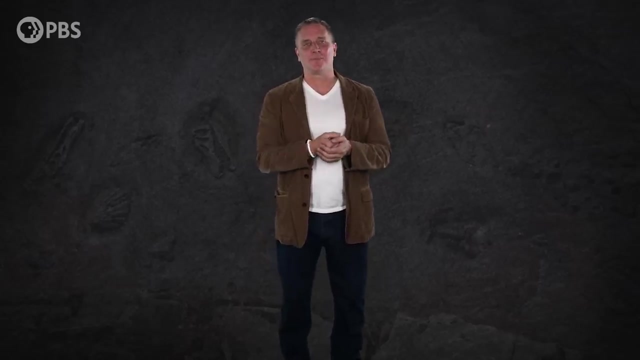 between humans and Neanderthals Stretching back tens to hundreds of thousands of years. those Neanderthals had already been changed forever by the introduction of human DNA into their gene pool long ago, Thanks to our fellow humans. this month's Eontologists 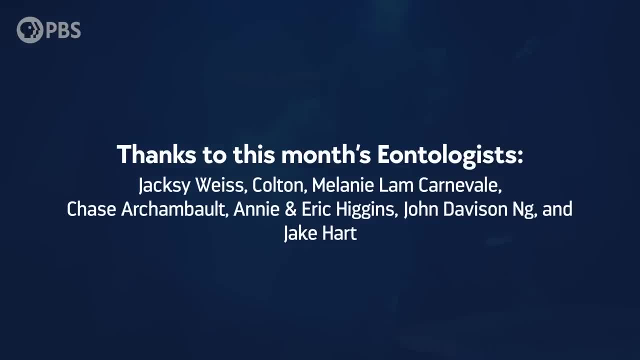 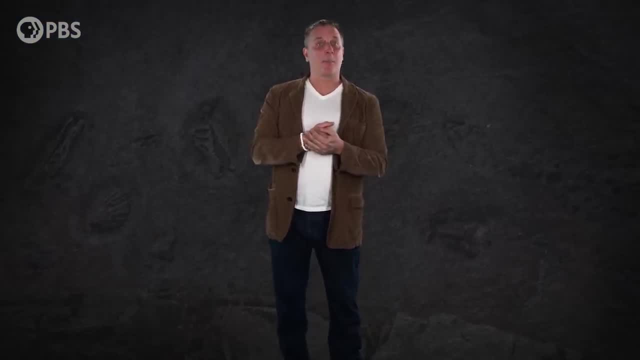 Jack C Weiss, Colton, Melanie Lam, Carnivale, Chase Archambault, Annie and Eric Higgins, John Davison Ng and Jake Hart. By becoming an Eonite at patreoncom- slash eons- you can get fun perks like submitting.